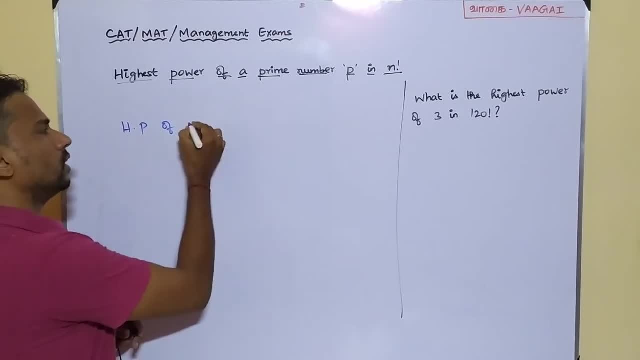 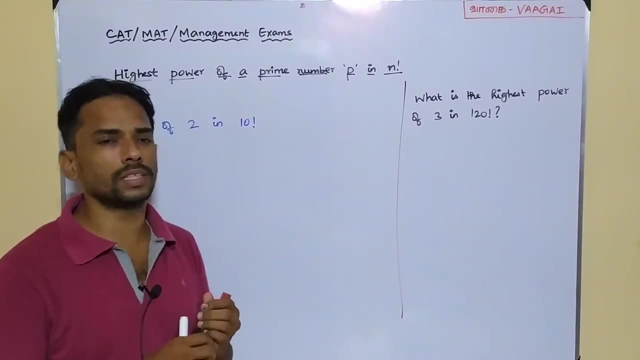 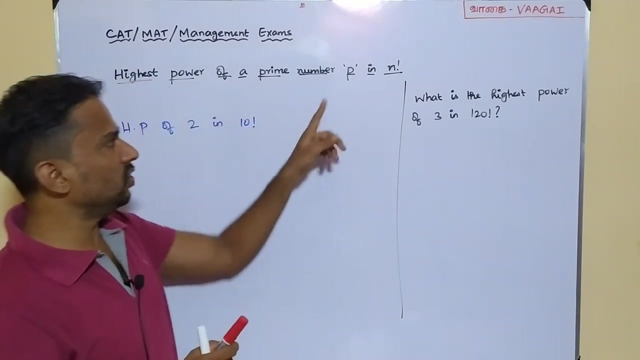 let me just write it in a short form: What is the highest power of the number 2 in 10 factorial Suppose, if I want to solve this question? So here, in this case, our value of n is 10 and the value of p is 2.. And here be clear, the value of p must be a prime number. Yes, And yeah, of course. 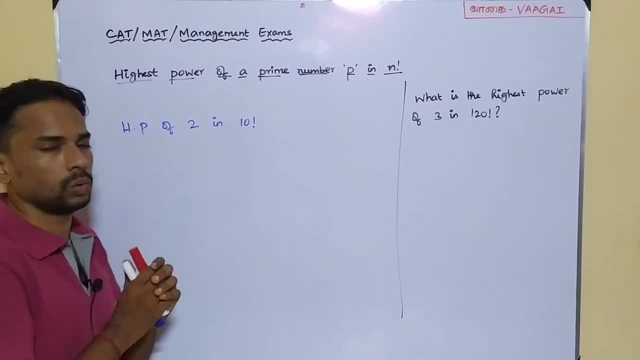 our question is also in the same structure: highest power of 2 in 10 factorial. And how are we going to solve this question? That is going to be the objective. So if you see here in this 10 factorial, we know what is factorial. Factorial of a number is 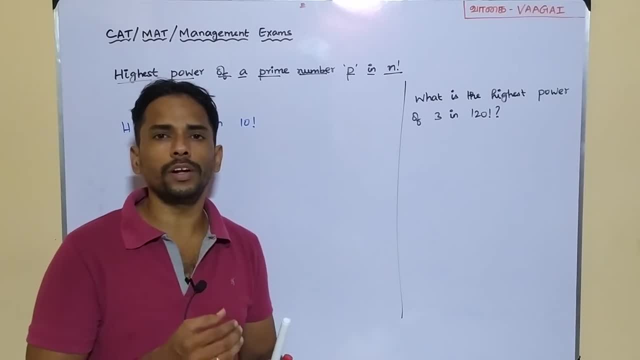 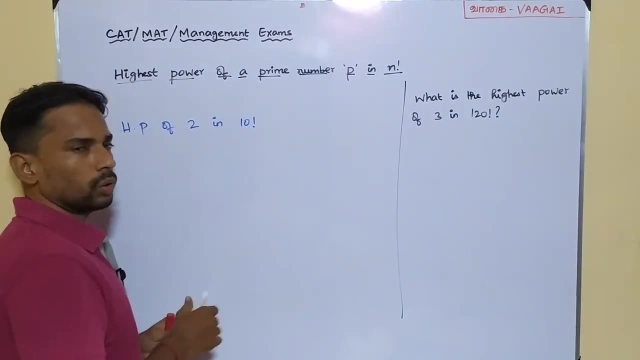 nothing but factorial of any natural number is going to be the product of all the numbers from 1 to n. That is what is factorial, right? Yes, So in that case here we have got 10 factorial. So this 10 factorial will be nothing, but it is going to be the product of all the natural 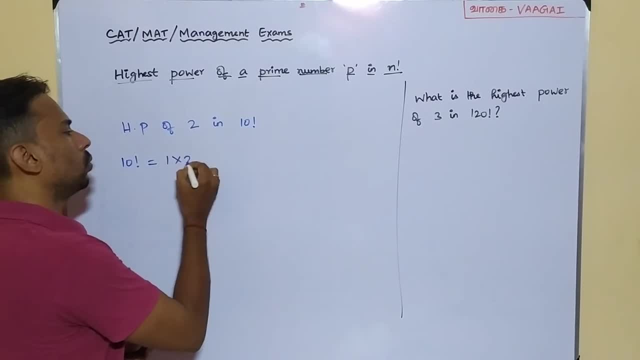 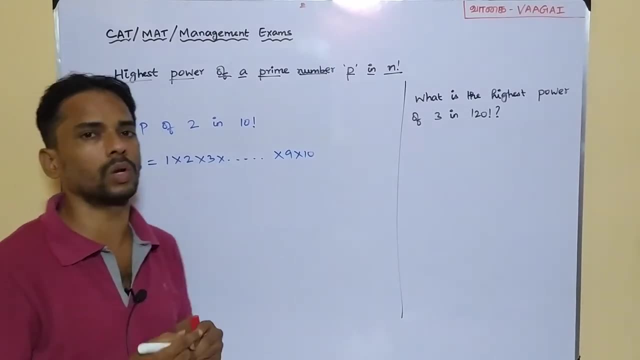 numbers from 1 to 10. So that is 1 into, 2 into 3 into, and so on till 9 into 10.. This is going to be the expansion of 10 factorial, And here we are supposed to find what is the. 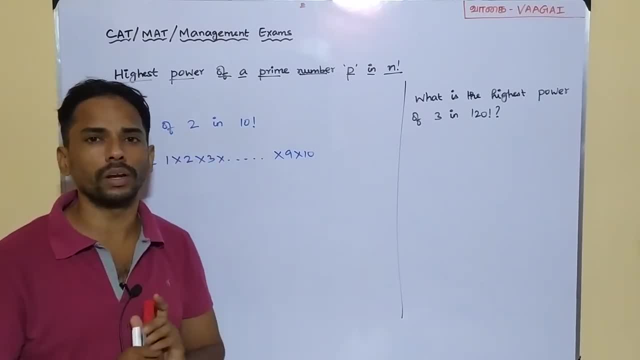 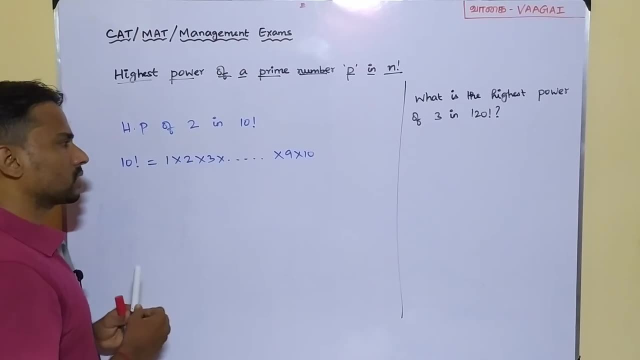 highest power of 2. we have got inside this 10 factorial right, So we will try to use the basic approach in order to solve this problem. So what I am going to find here is: I am going to see wherever I have got 2 here in this entire product And also I am going to find out the highest power. 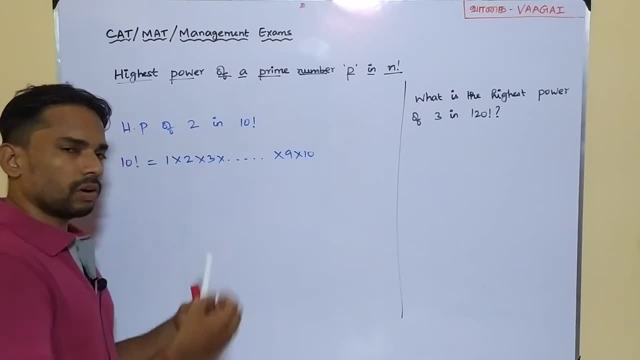 I mean the maximum power available, maximum power of 2 available here in this product. That is going to be the objective. Yes, So, if you keenly observe, 2s will be available only in even numbers, Is it or not? So, if I consider this product, 1 into 2. 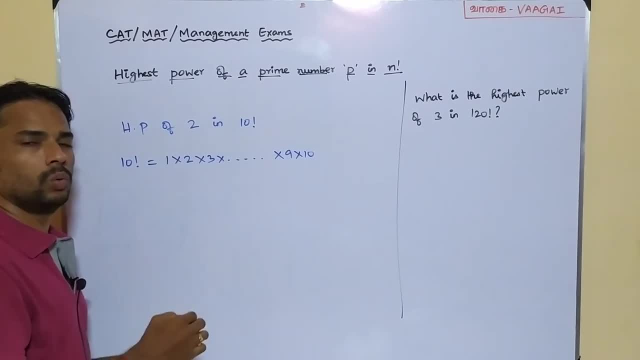 into 3 into, and so on up to 10,. I will definitely have 2 only in the even numbers, And so I need not consider any of the odd numbers here, Because it is mere waste of time if we just sit and examine whether we will be having 2 inside a 1, or inside a 3 or inside a 5.. 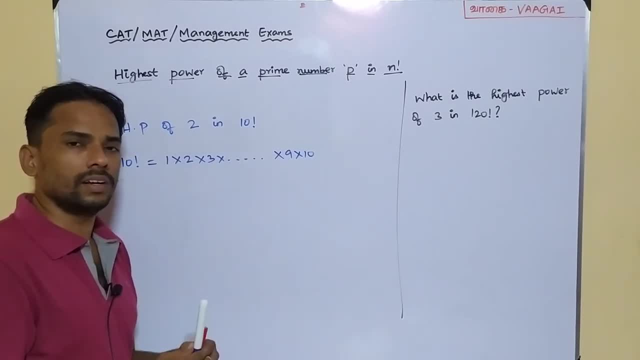 So, because I will definitely say that, I can easily say that, definitely say that I will never have 2 inside the odd numbers. I will have 2 only inside the even numbers. So let me just pick only the even numbers which I have here. Yes, ready Shall, we do that. So if I try to do it, I will have 2,. 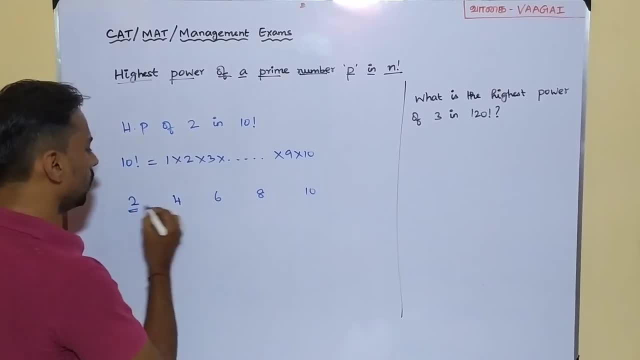 4,, 6,, 8, 10.. Only these are going to be the even numbers, And we can assure that 2 will be there only inside these 5 numbers. And now the next task is to see what is the highest power of 2 available in each of these numbers. Shall we do that? Yes, 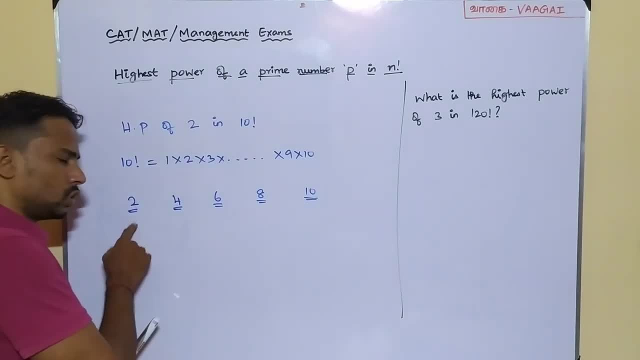 we will start from this 2.. So it is very easy to say, inside this 2, there will be only 1, 2. That means I can have 2 power, 1 maximum inside this 2.. Coming to this 4.. So this 4, inside that 4,. 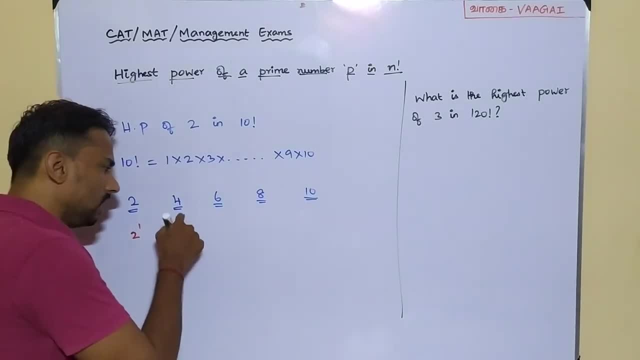 I will be having 2 2s, Is it or not? So that is inside this 4, I have got 2 square. So that is, I have got 2 2s here. Or even I can say that: 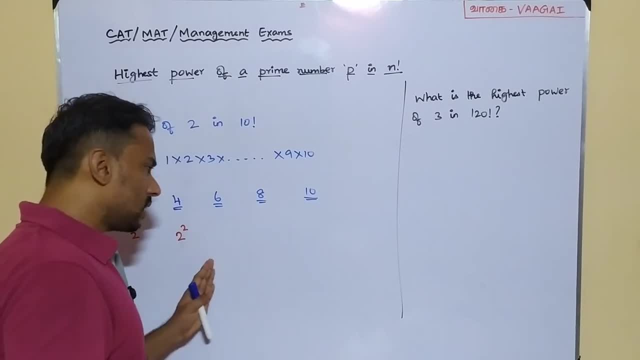 I have 2 power 2 inside this 4.. Same way, let us examine the same thing here in all these remaining numbers also Coming to the 6. So inside the 6 again, we will happen to get only 1, 2, because I 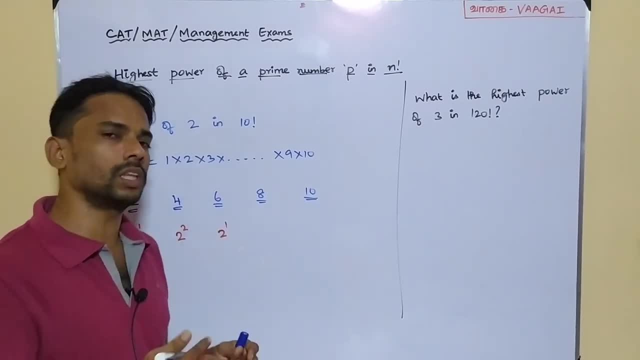 will have only 2 power 1 inside the 6.. Because 6 is nothing but the product of 2 power 1 into 3 power 1.. Is it or not? So in that case we will have 2 power 1 alone here in this 6. And coming. 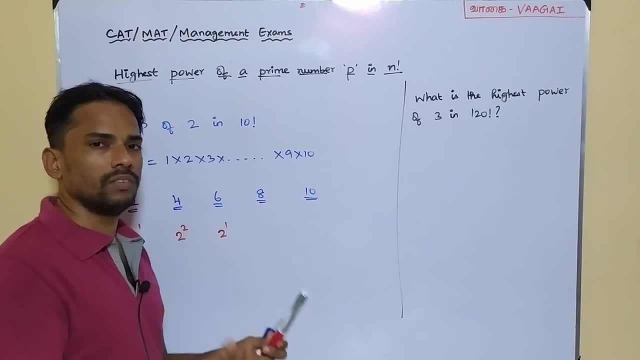 to this 8.. So inside this 8, a stone is going to be 2 power 1.. So inside this 8, I have 2 power 1 here. So that means we have got 3 2s. So we have got 2 power 3 here, because 8 can be expressed as: 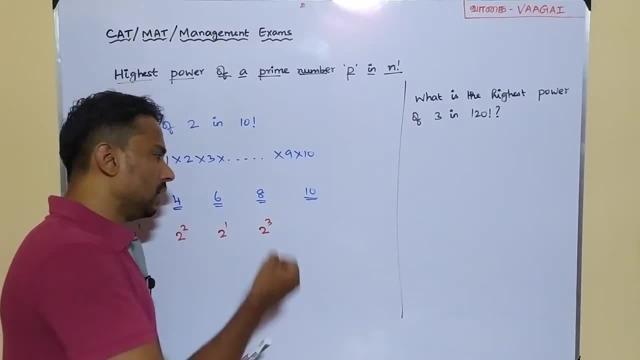 2 cube, So that means maximum 2s available. inside this 8 will be, there will be 3 2s available, So 2 power, 3.. And again, coming to 10, there again we will have only 1, 2. That is I can have maximum. 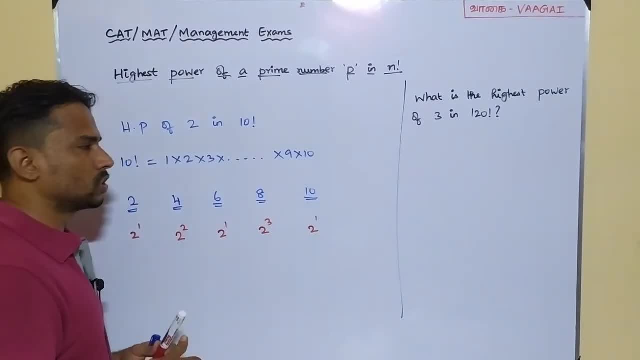 2 power 1 inside that 10.. And now our objective is to find how many 2s are there in this entire product. I mean 10 factorial. So in that case we have got 2 power 3 here. So we have got 2 power 3. 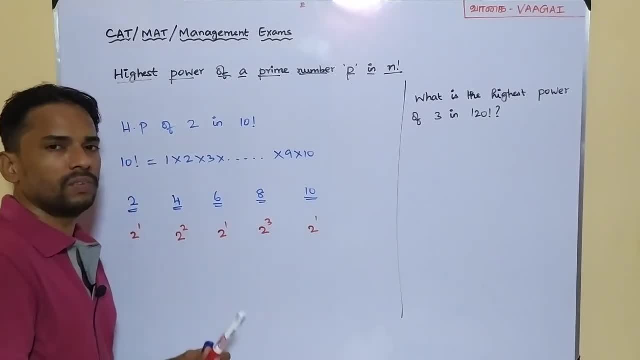 here. So in that case we can just take all these numbers, products, and that will give us the maximum power available in 2.. Is it or not? So, shall we do that? So in that case, if I multiply all these numbers, I will have the chance of getting the maximum number of 2.. I mean the maximum power of. 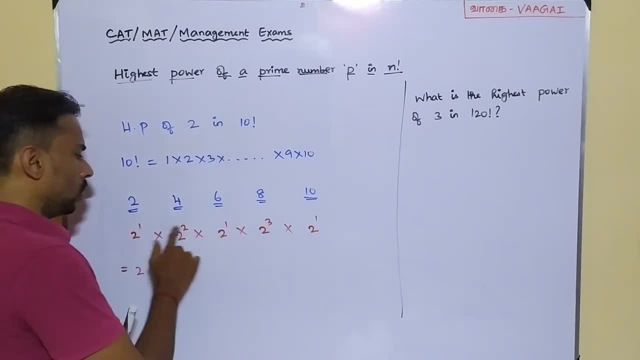 2 inside 10 factorial. Let us do that. So 1, 2, 1, 3, 1.. So when we just multiply all these numbers, our bases are same, but powers are different. So in that case we can just add up all the. 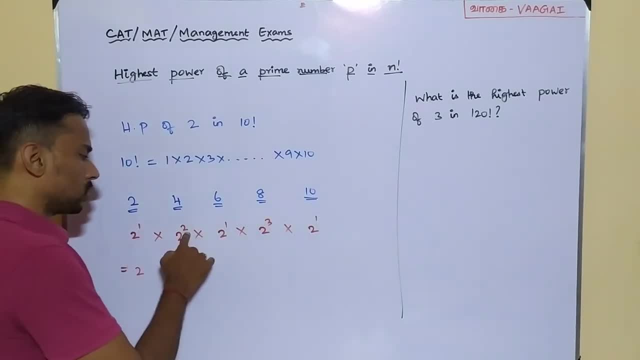 powers, Is it or not? So if we try to do that, we will be getting 1 plus 2, which is 3.. 3 plus 1 is 4.. 4 plus 3 is 7.. 7 plus 1 is 8.. So in that case we have got 2 power, 8 inside this, 10. 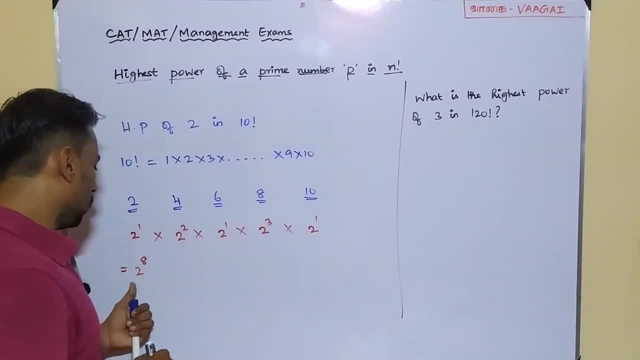 factorial. That is the result we can arrive with. So we have got 2 power 8.. So that means the maximum or the highest power of 2 available in 10 factorial is nothing but 8.. So because we have got 2 power 8, that is, we can collect maximum 2 power 8.. 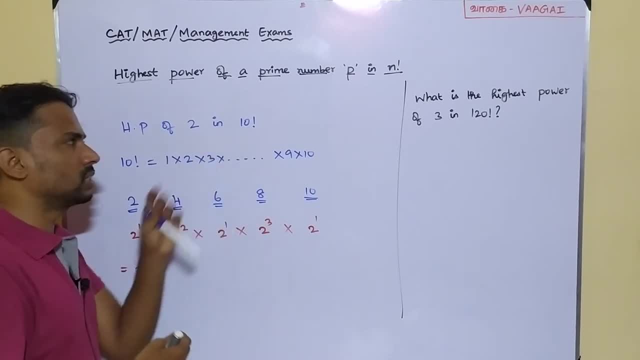 Or I can say: we can collect maximum 8 2s from this 10 factorial. That is the meaning. So that is what stands for this highest factor, highest power of 2 in 10 factorial. That is it So. but what if we get some bigger numbers? Let us see our question. We have got 120 factorial, Can you? 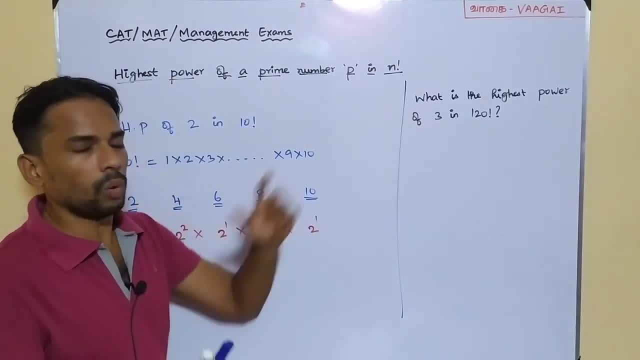 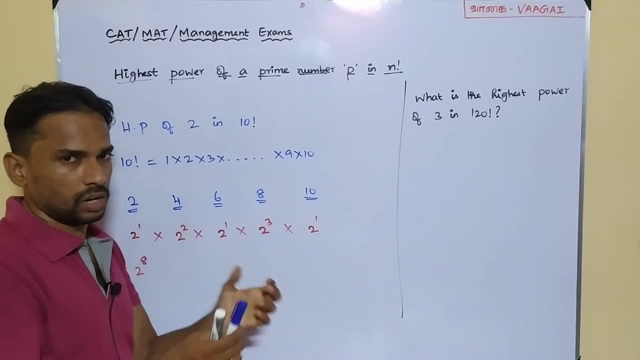 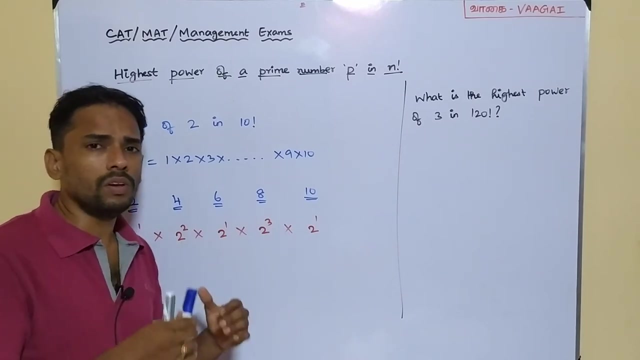 even imagine doing the same process for 120 factorial. Is it going to be that easy, like we did here? Since our number here is a smaller number comparatively a smaller number, just 10 factorial. We are easily able to do this answer by a basic approach. But what if we are given a? 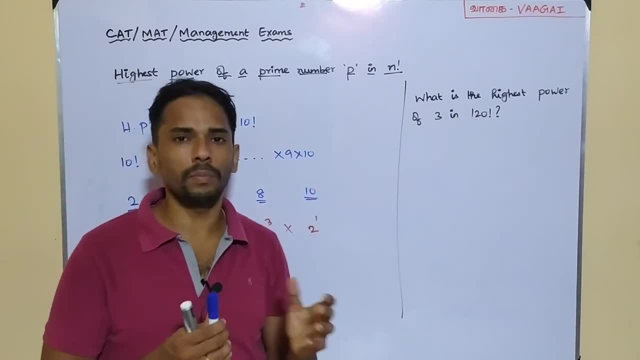 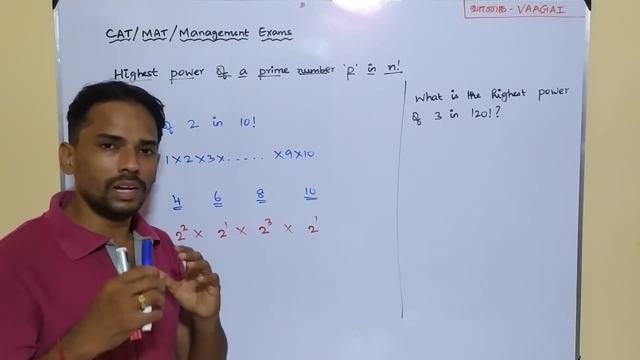 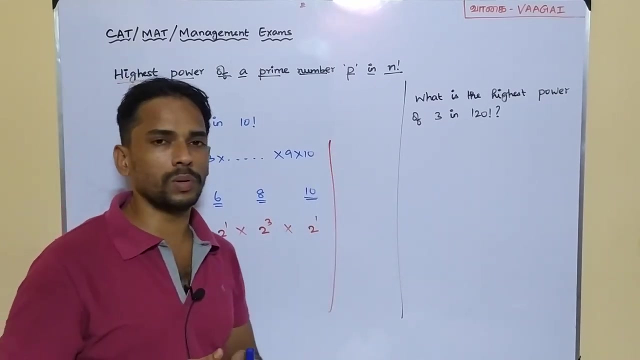 very big number, or a number even bigger than this. What can be done? So, for that is what we are going to execute- a very easy shortcut, and we are going to solve the same problem. Let us see how that shortcut is going to work. So, in order to execute that shortcut, I think this small space is enough. 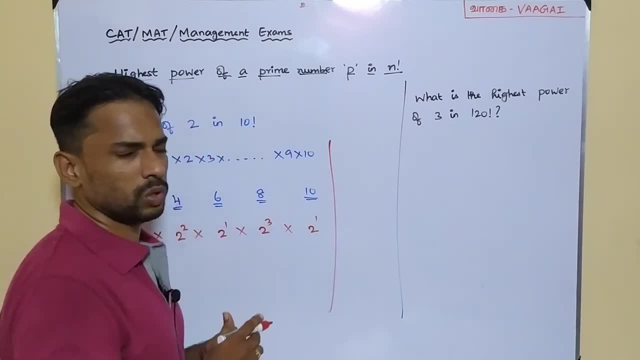 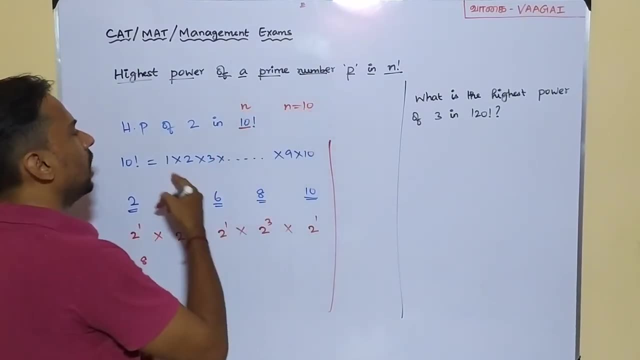 for us. So, yes, how that shortcut is going to work. It is going to be a very simple process, So let us see how that shortcut is going to work. So let us see how that shortcut is going to work. So here our n value is 10.. So here our n value is 10.. And here, highest power of 2, our p value is 2.. So 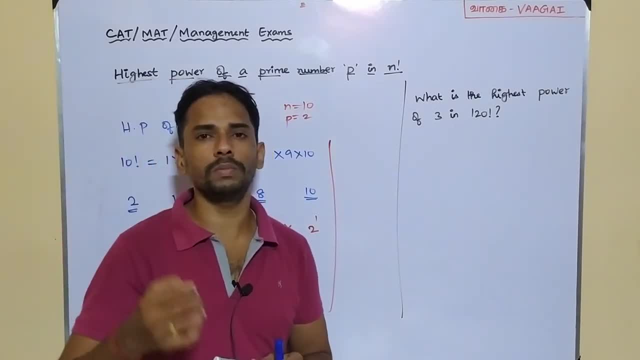 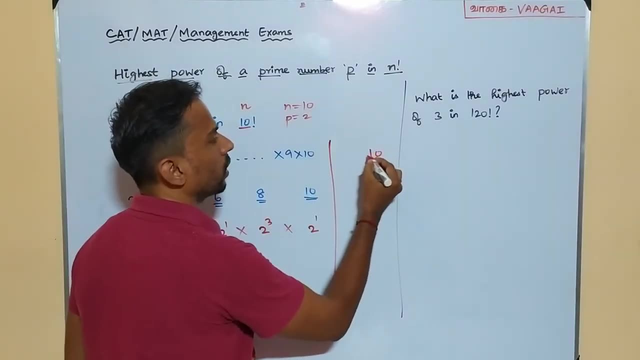 in school days we used to do step division. right, The same step division is what, now again, we are going to employ here. So see how I am going to start with. I am going to start with this 10.. Okay, start with this 10 and try to do repeat factorization or step division with 2.. Yes, 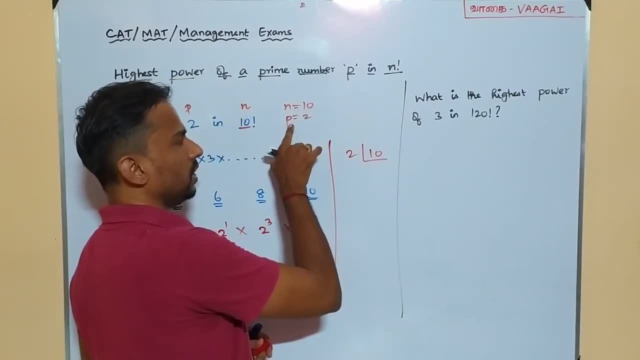 ready. So I am going to start with 2 because our highest power, we need to find the highest power of 2 only here. So that is the reason I am just going to divide it by 2.. I am going to do repeated: 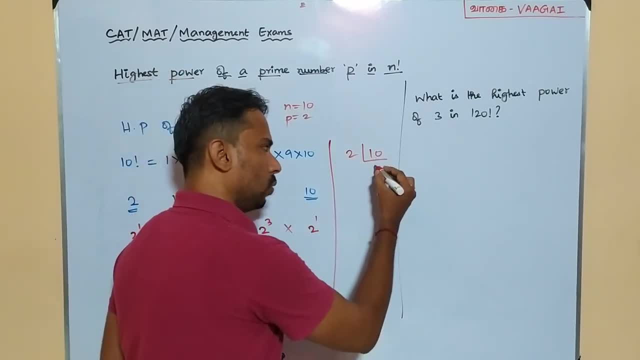 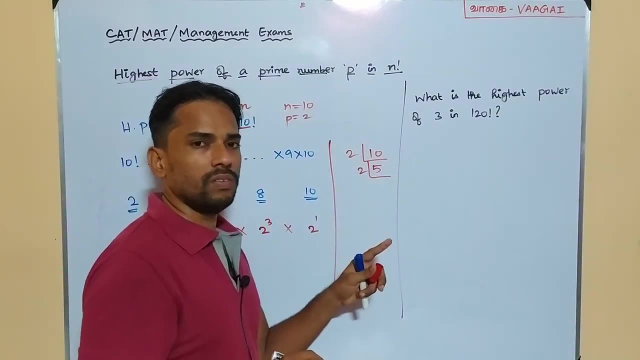 division by 2.. Yes, 10 divided by 2, I can do exactly 5 times. Again we have got 5.. Again, take it 2, divide it by 2.. So 5 into how many times will it go? It can go for 2 times, right. 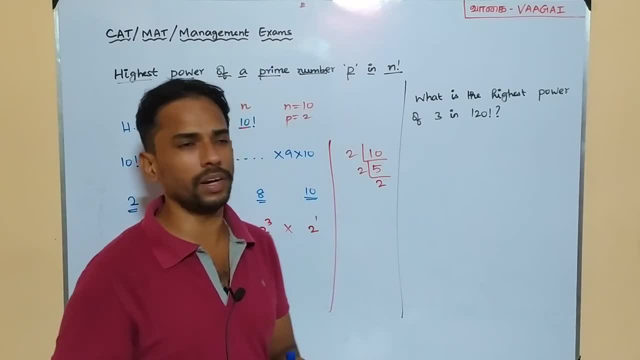 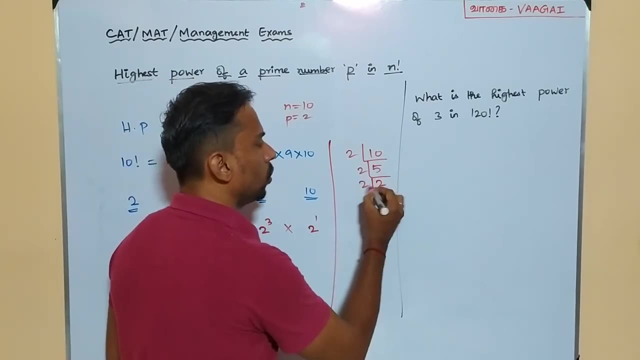 Of course there will be a reminder: 1.. But just do not worry about the reminders, Just take only the quotient. We just need how many full numbers are there. That is why, So 2 and once again 2, I can go for 1 time. Yeah, I can stop here, because we have got a number which is 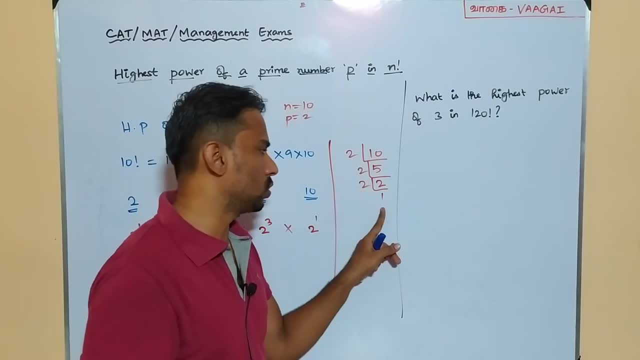 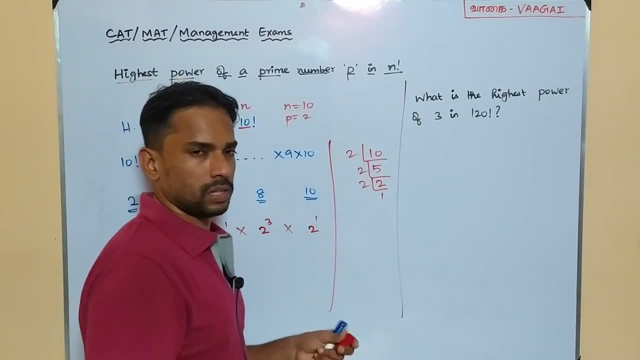 lesser than the number with which we are dividing. So we have got 1.. So stop there. So I started with 10 and just doing repeated step division. I got these steps right, So now your process is over. Now all you need to do is just strike out the first number. I mean the number. 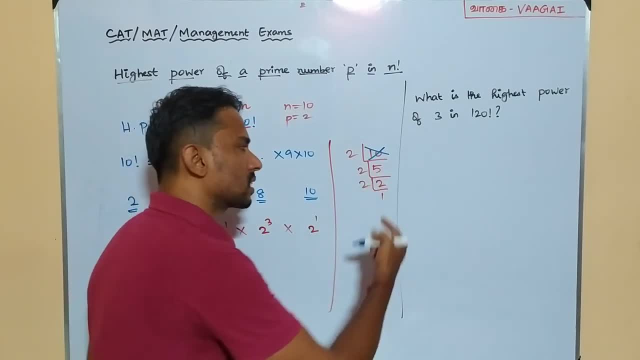 with which you started. Just strike out that number and just consider the other numbers alone: This 5,, this 2, this 1.. Just add all these numbers, 5 plus 2 plus 1, and that gives you the answer 8.. And that is. 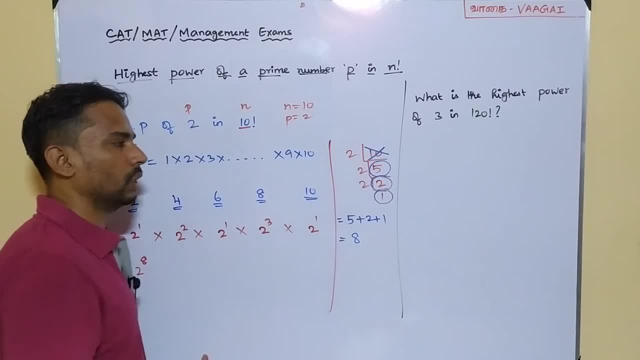 going to be the answer for what is the highest power of 2 in 10 factorial. I hope the process is clear to you. So this is going to be the approach, the basic approach, with which we can solve the problem. In order to understand the concept, we can go refer this method, But all 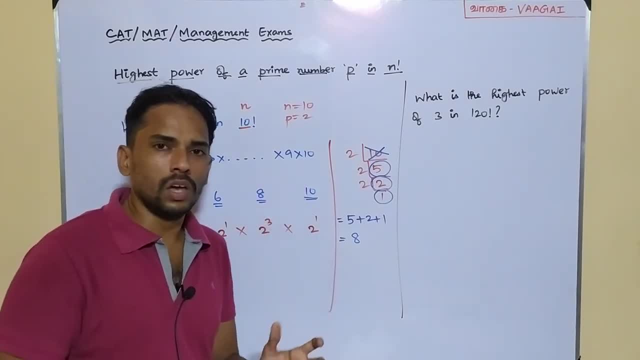 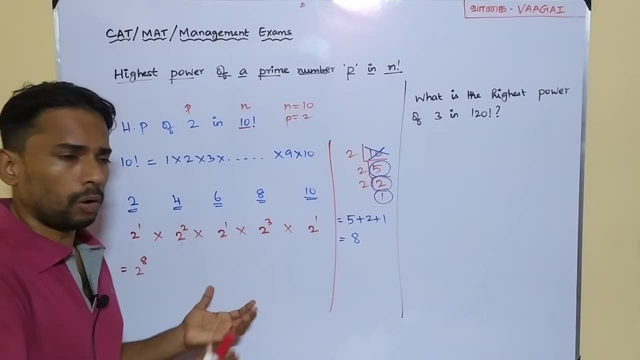 the time, you cannot do the problems using the same method, since if we get some bigger number, it would be a great challenge, or you would see, to solve the problem using the same method. So, in order to complete your problem in a very easy way, 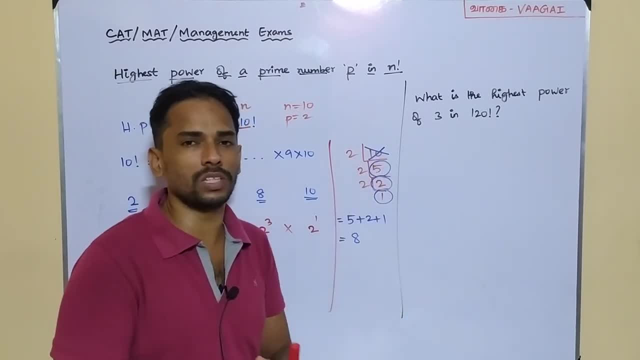 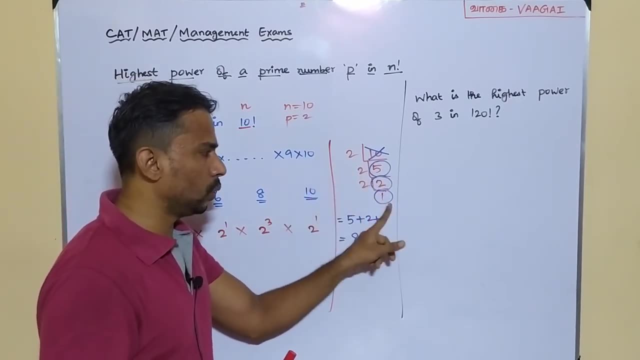 in an efficient way. you can just go for this repeated step division process. This looks very cool, right? So 10, you are repeatedly dividing it by 2.. So 5 times again 2,. 2 times again 2,. 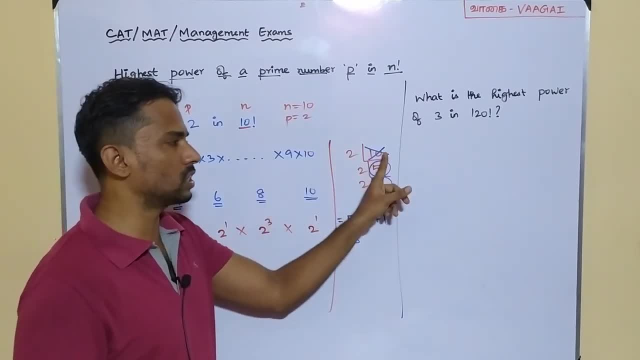 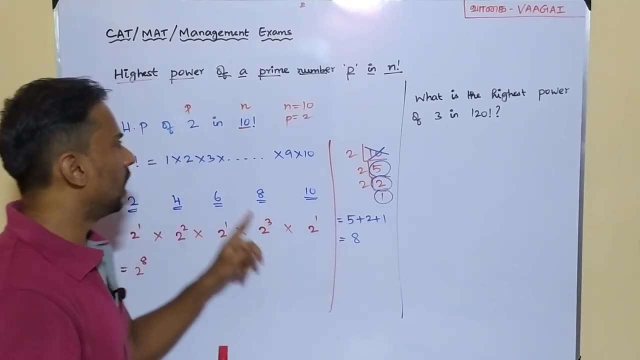 1 times. That's it. Just eliminate the first number, I mean our n value, Just eliminate the 10.. Take only the other numbers, So 5 plus 2 plus 1. That gives you the answer 8.. So that means the. 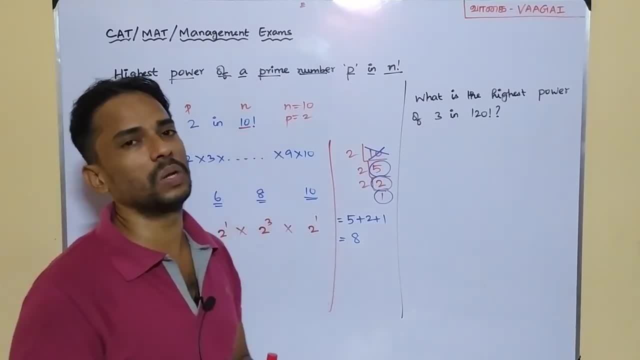 highest power of 2 in 10 factorial is going to be the highest power of 2 in 10 factorial, So that's going to be 8.. That's it Now. I think the process is clear to you. Now let's try to solve the problem. 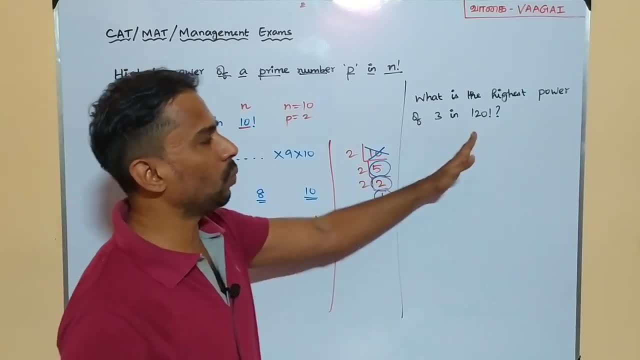 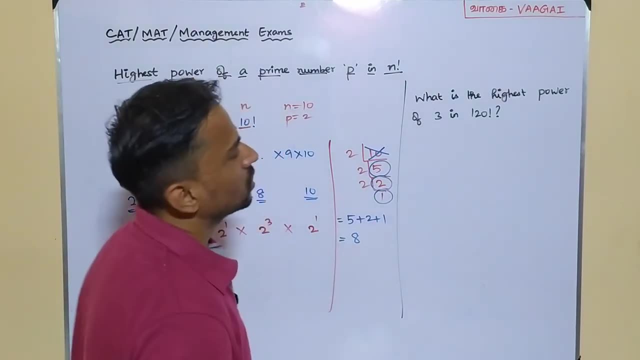 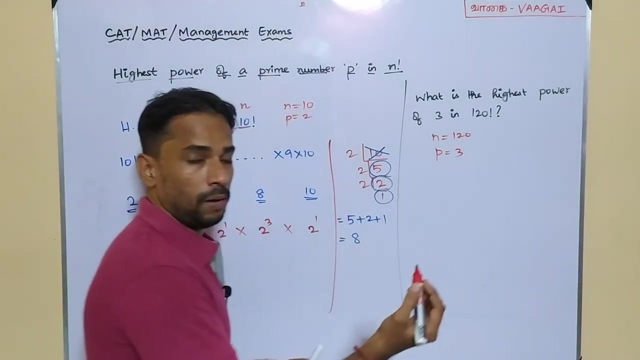 which we have got here. What is the highest power of 3 in 120 factorial? I think we can directly go with this step. division method itself: Yes, if you are ready, we can start. So yes, we'll begin. Our n value here is 120 and our p value here is 3.. Is it or not? So in this case, we have to start. 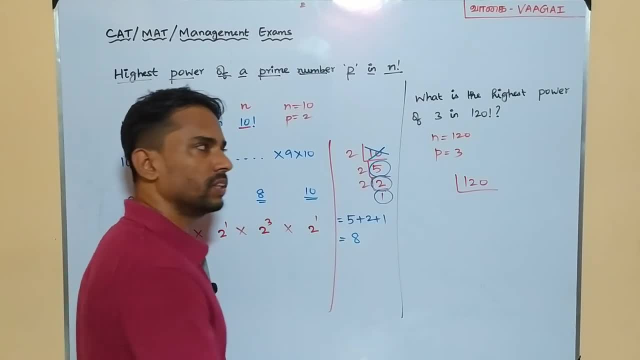 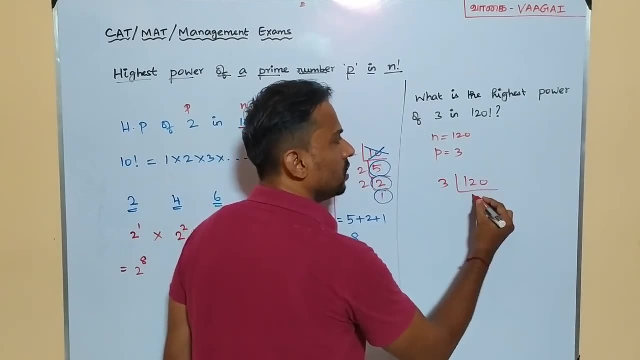 with 120, and I'm going to repeatedly Do my division with the number 3, because here our p value is 3. So start your division with 3. So 120 in 3. It's exactly 40 times, And once again go for 3. So 40 in 3. We can go up to. 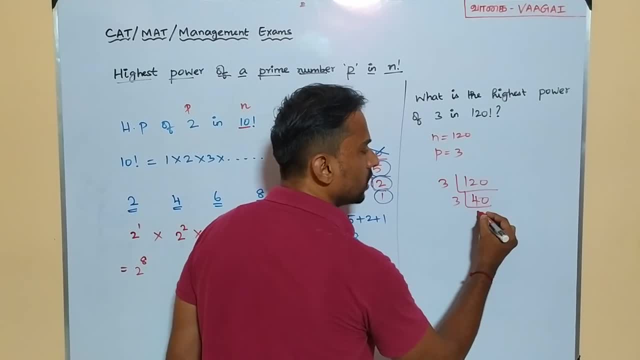 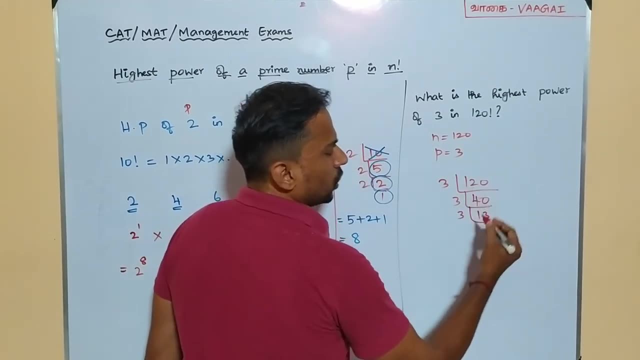 13 times, Is it or not? Because 3 13ths are 39.. So we can go up to 13 times, As I told, only the quotient is important- And once again go for 3.. So 3 4ths are 12.. So we can go up to. 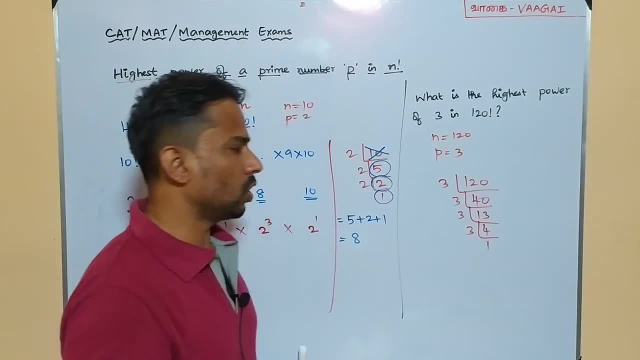 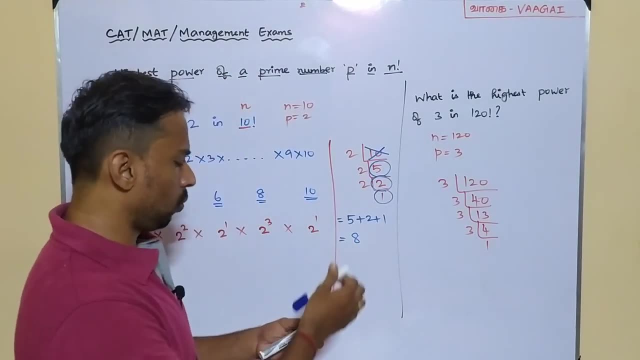 4 times And once again, 3 1ths are 3.. Yes, that's it. So we can't proceed further because we have got a number which is still lesser than our number with which we are dividing, And, as usual, what else we can do is we'll just eliminate our first number, 120, because 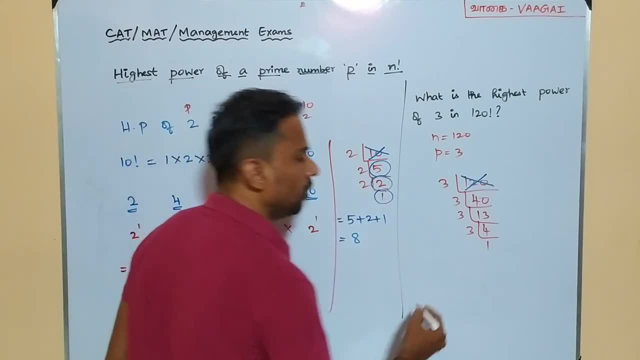 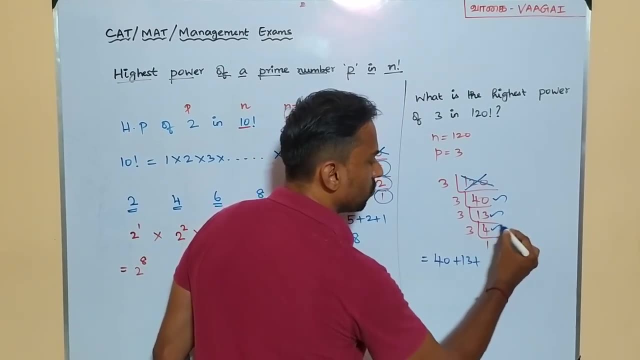 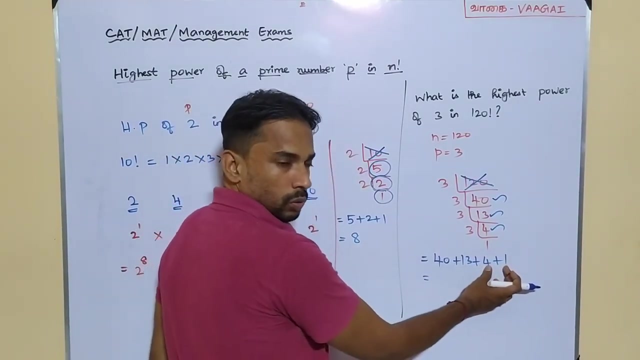 that's a number from where we started. So eliminate that number and we have to add all the other numbers. That is this 40.. Yes, then this 13 plus this 4, then plus this 1.. So this would give you 40 plus 13 plus 4 plus 1.. This will be a 5.. 4 plus 1 is 5. 5 plus 13 will.